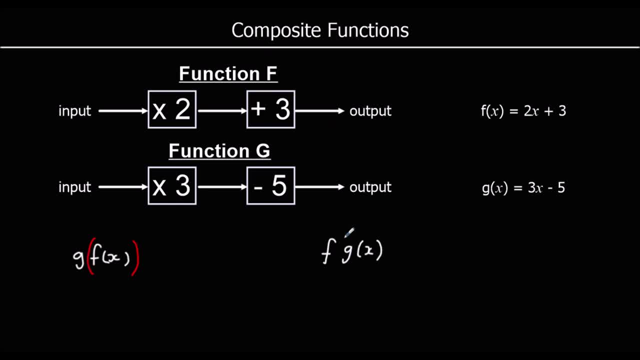 The same as putting the entire g function into f. So with g, f of x, we're taking the entire f function, which is 2x plus 3. And putting it into g. So we're changing x, we're changing the input for the g function to 2x plus 3.. 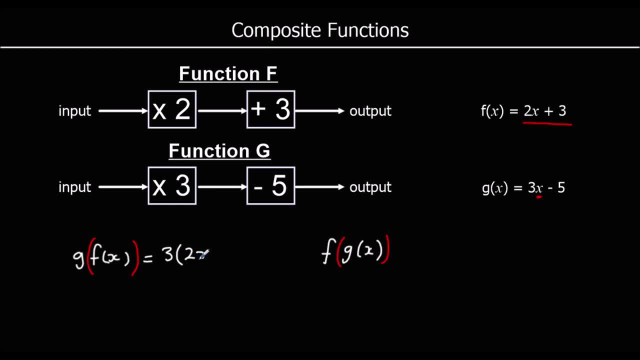 So we're going to have 3 times 2x plus 3, take away 5., Which we can expand the bracket, So 6x plus 9 minus 5. Or 6x plus 4.. So what we're saying is if we run the f function. 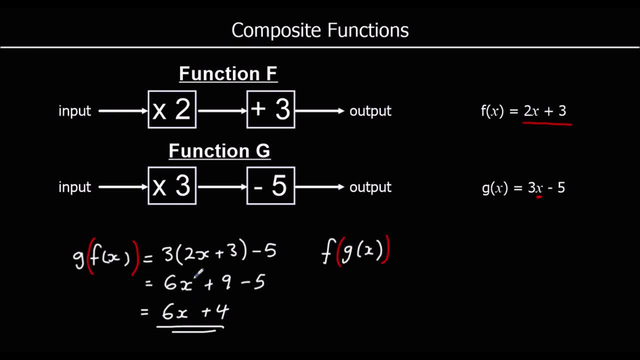 and then the g function. that's the same as multiplying by 6 and then adding 4.. If we run the g function first and then the f, that's the same as taking the entire g function and substituting into f. So it's 2 times 3x minus 5 plus 3.. 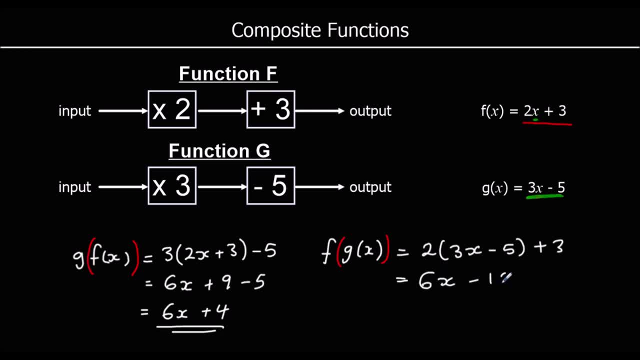 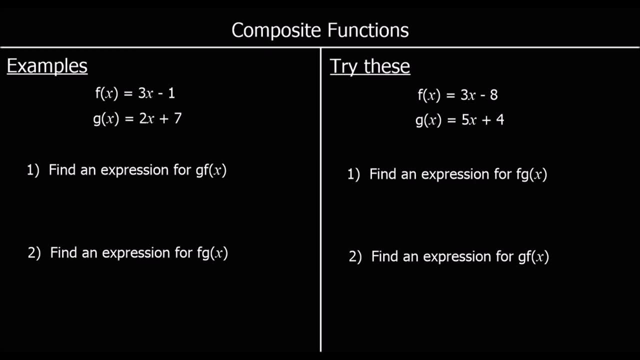 So expanding the bracket, that's 6x minus 10 plus 3. Or 6x minus 10 plus 3. Or 6x minus 7.. Let's look at some examples of this. So we've got two functions, an f function and a g function. 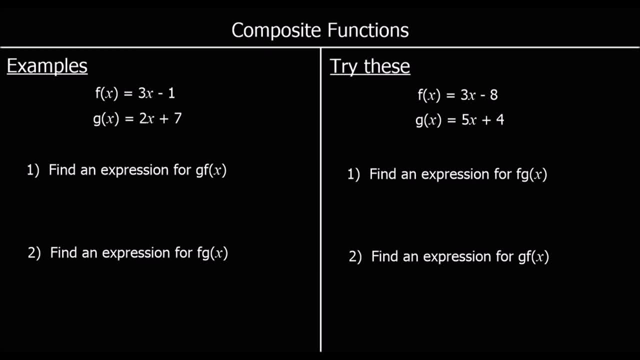 And we're being asked to find the expression for g, f of x. That means putting our f function into g, That our total f function, all of our f function. so 3x minus 1 into g, So g of 10.. 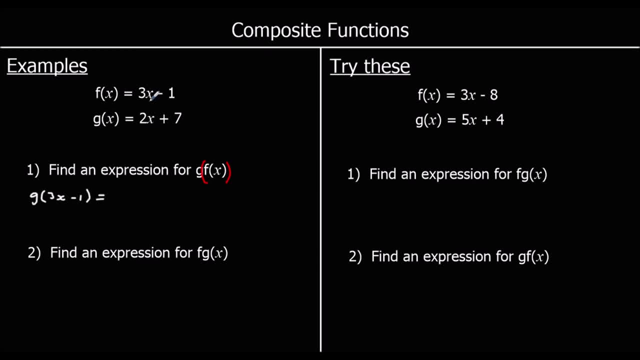 3x minus 1.. So we're changing x into 3x minus 1.. So it's 2 times 3x minus 1 plus 7.. So expand the bracket 2 times 3x is 6x. 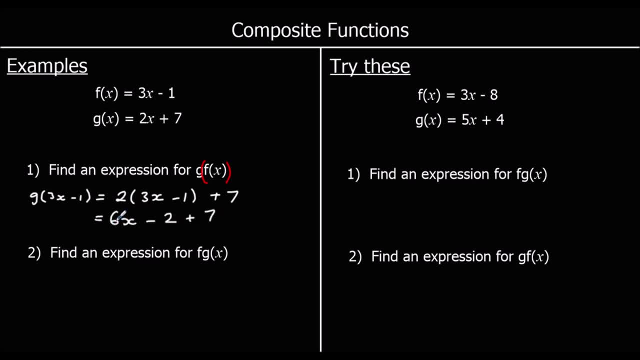 2 negative 1s and negative 2.. So we've got 6x minus 2 plus 7, which is 6x plus 5.. So g? f of x is 6x plus 5.. How about f? g of x? 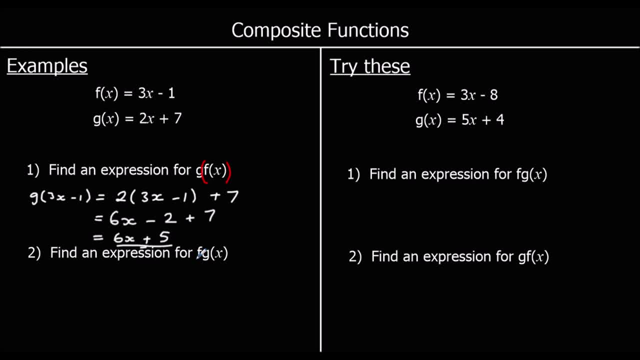 So taking the g function and putting it into f, So the g function is 2x plus 7.. So we're going to do f of 2x plus 7. Which is 3 times 2x plus 7 minus 1.. 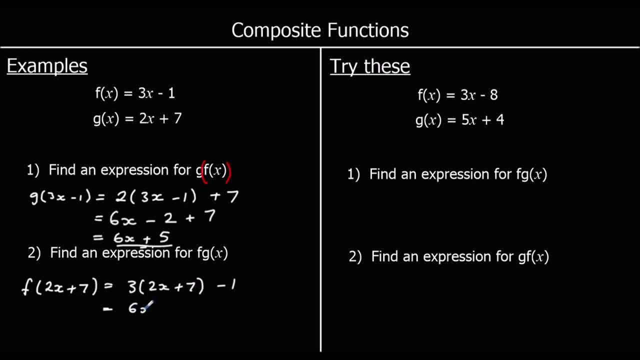 So, expanding the bracket, We've got 6x plus 21.. 6x plus 21 minus 1, which is 6x plus 20.. Okay, two for you to try, So give them a go. The first question: find an expression for f, g of x. 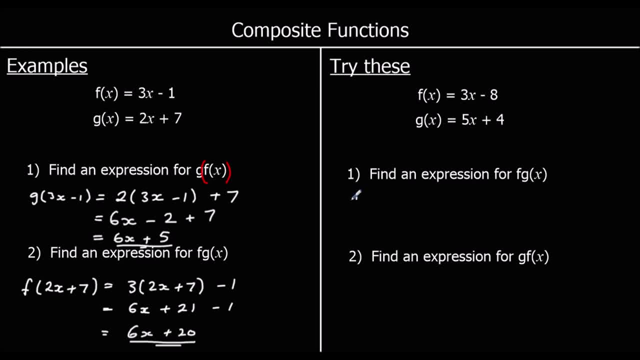 So putting g into f, So it's f of 5x, 5x plus 4.. So that's 3 times 5x plus 4 minus 8.. If we expand the bracket 3 times 5x is 15x. 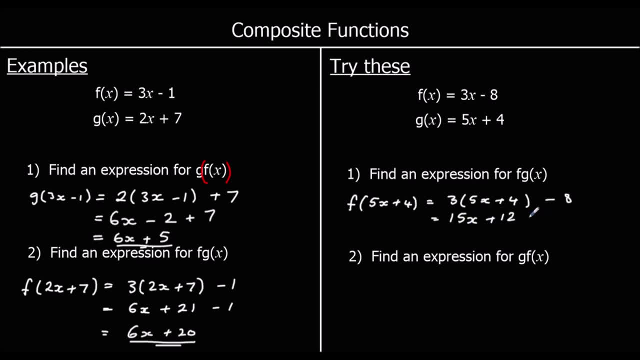 3, fours are 12.. So we've got 15x plus 12 minus 8, which is 15x plus 4.. And we've got g, f of x. So putting f into g, So g of 3x minus 8.. 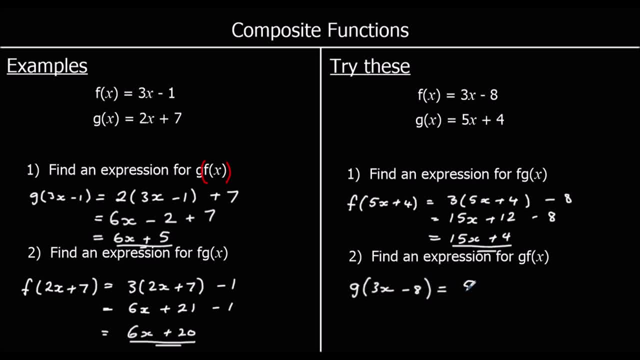 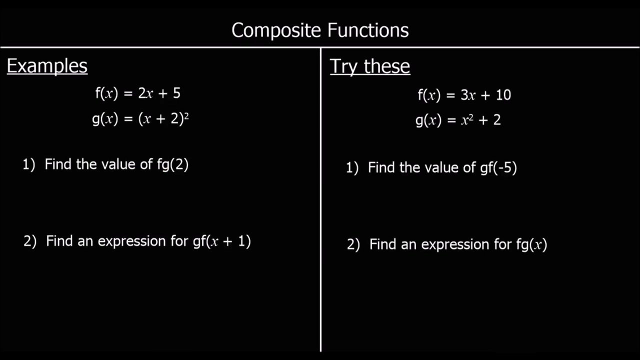 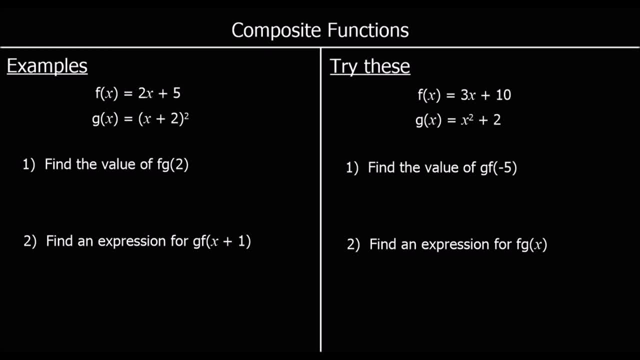 Thank you, Thank you, Thank you. Two more questions here. We've got an f function and a g function still. The first question this time says: find the value of fg of 2.. So we're putting 2 into g and then putting that into f. 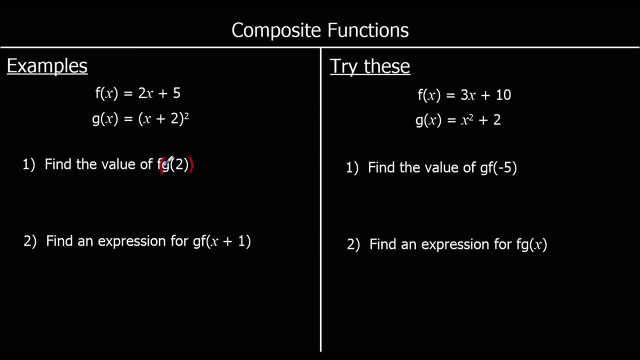 So we're going to put 2 into g, first find out what that is, and then we're going to put that into our f function. So let's do g of 2 first, which is going to be 2 plus 2 squared. 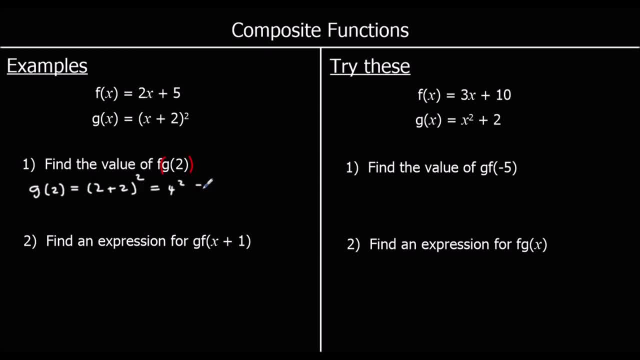 2 plus 2 is 4, so 4 squared, which is 16.. So we're putting 16 into our f function. So we're going to do f of 16.. So g of 2, we know that's 16 now, so we've changed that to 16.. 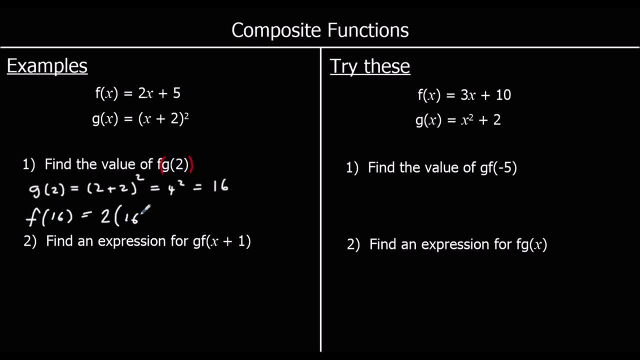 f of 16 is 2, 16s Plus 5, which is 32 plus 5, 37. Question 2, find the expression for g f of x plus 1.. So we're going to put x plus 1 into f and then put the answer to that into g. 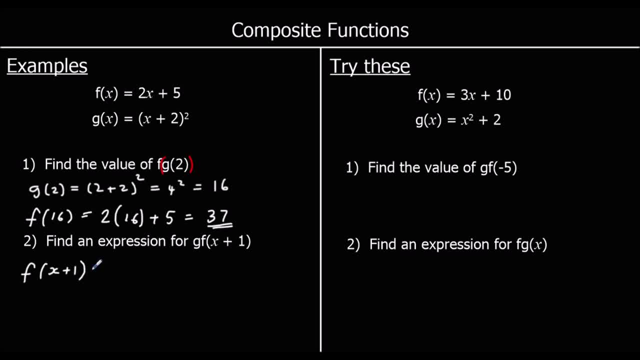 So let's work out f of x plus 1, which is going to be 2 times x plus 1 plus 5.. Expanding the bracket, so we've got 2x plus 2.. 2x plus 2 plus 5 is 2x plus 7.. 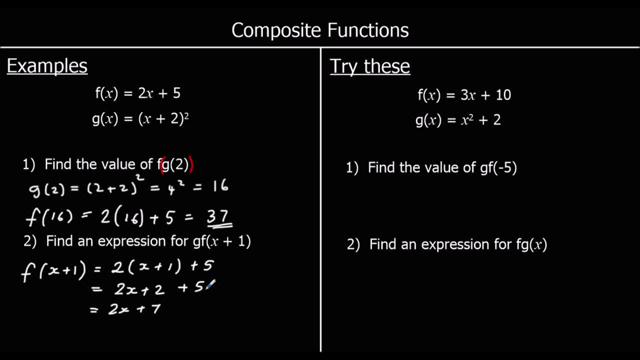 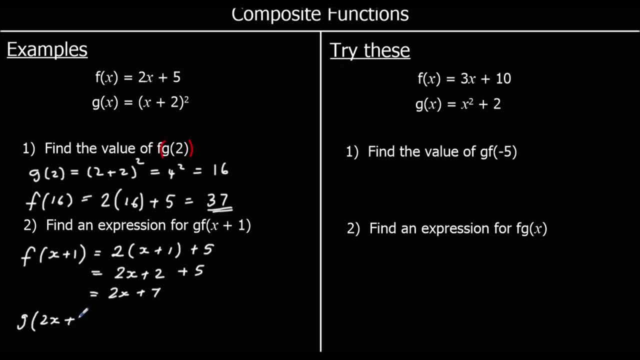 So f of x plus 1 is 2x plus 7.. We're going to put that into g, So we're doing g of 2x plus 7. And g is x plus 2 all squared, So we're going to have 2x. 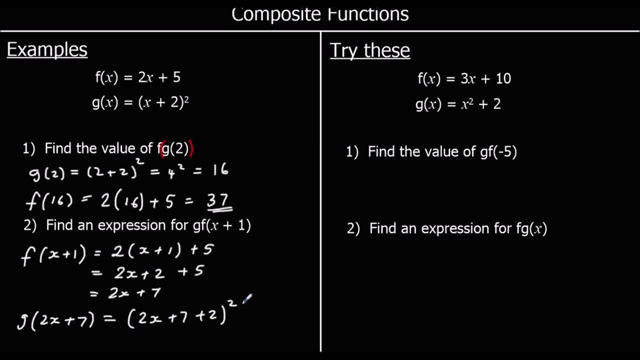 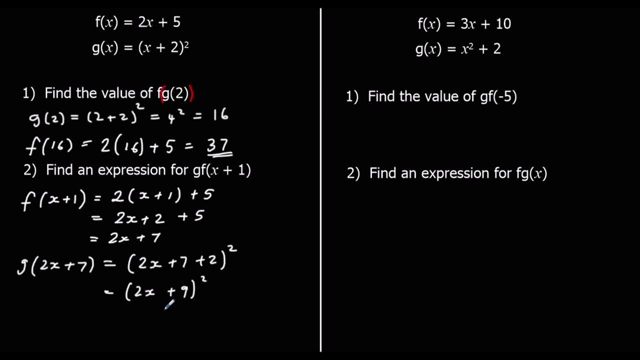 2x plus 7 plus 2 squared, which is 2x plus 9 squared. Squared means multiplied by itself. So we've got 2x plus 9 times 2x plus 9.. So we've got to expand the double brackets. 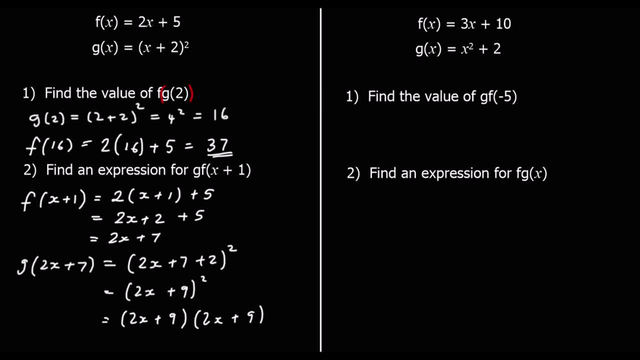 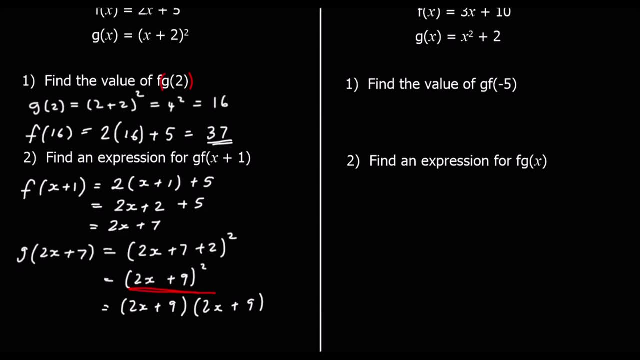 I suppose we could leave it as 2x plus 9 squared. We could leave that as our answer. That's a perfectly good answer. I will carry on just for fun. So 2x times 2x is 4x squared. 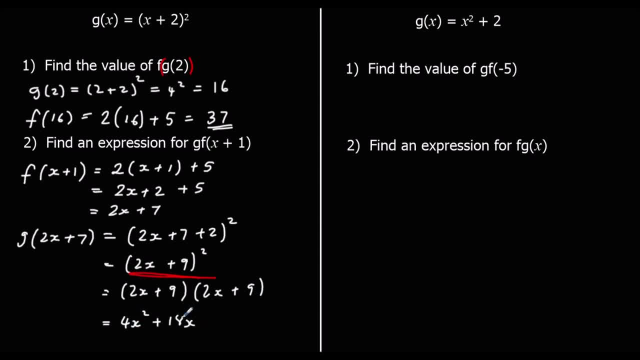 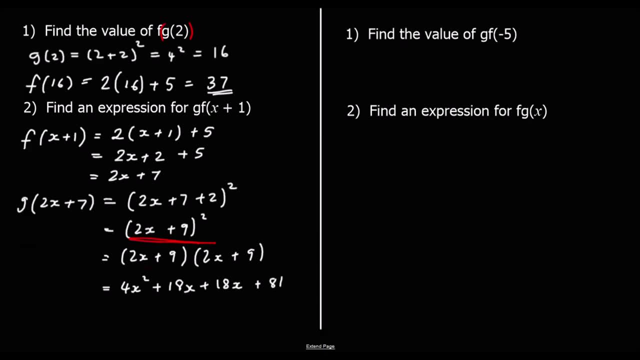 2x times 9 is 18x. 9 times 2x is 18x 9. nines are 81. So we've got 4x squared plus 36x plus 81.. As I said, we could have left their answer as 2x plus 9 squared. 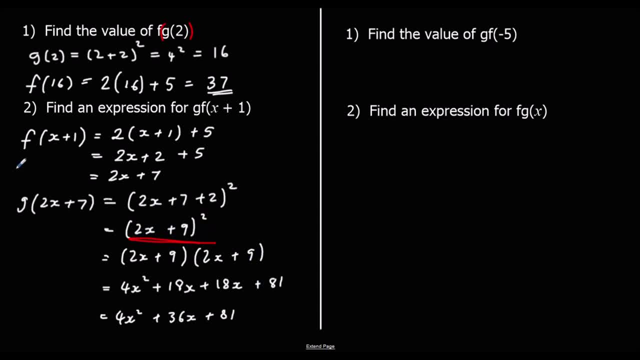 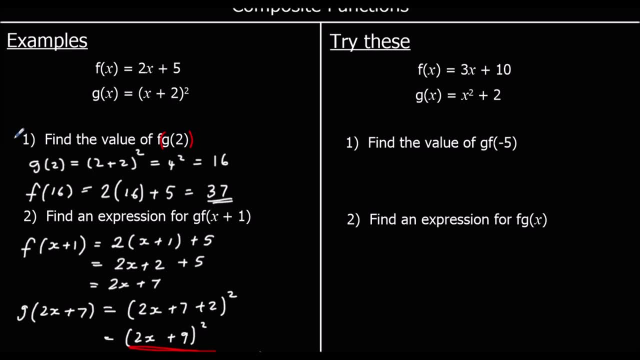 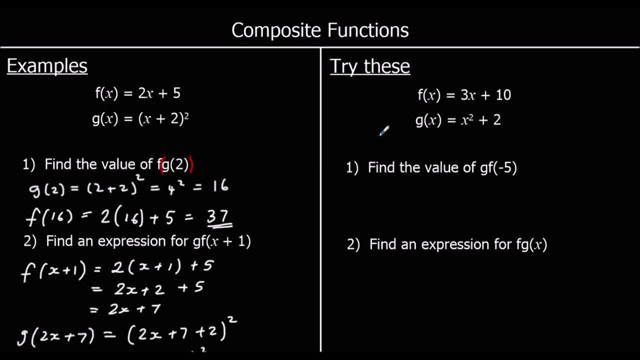 So give them a go. Question 1. We've got find the value of g, f of negative 5.. So let's put negative 5 into f, So we'll do f of negative 5 first. So that's 3 lots of negative 5 plus 10.. 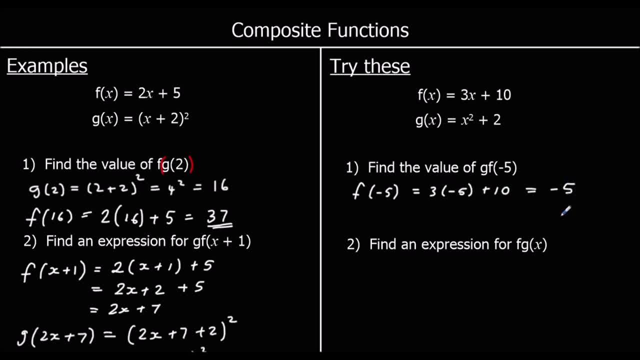 Negative 15 plus 10 is negative 5.. So we're putting negative 5 into g, Which is going to give us negative 5 squared plus 2.. Negative 5 squared is 25.. 25 plus 2 is 27.. 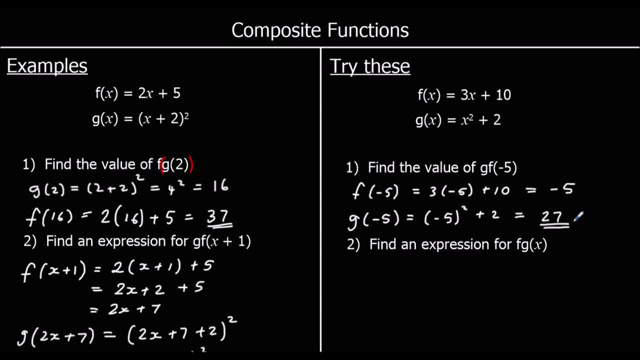 And question 2.. Find an expression for f, g of x. So we're putting g into f, So it's going to be the same as f of x squared plus 2.. So 3 times x squared plus 2 plus 10.. 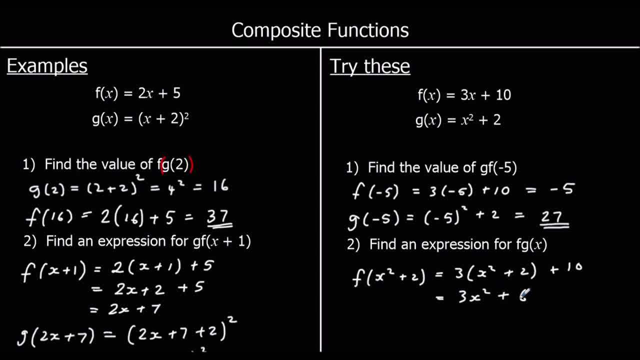 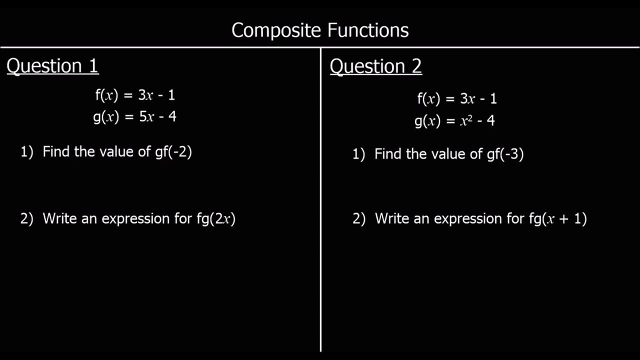 Which is 3x squared plus 6 plus 10.. Which is 3x squared plus 6.. Which is 3x squared plus 16.. And to finish up, we've got two more questions, So pause the video and give them a go. 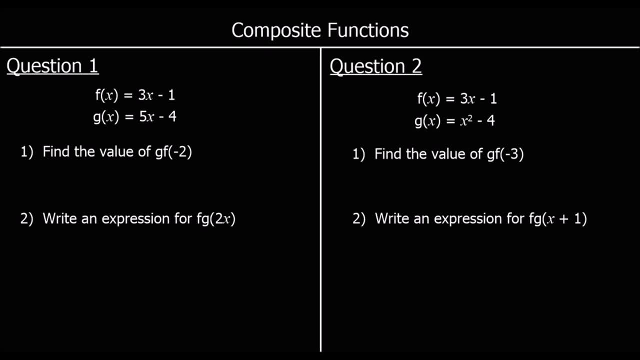 Question 1.. We've got our f function. f of x is 3x minus 1.. Our g function- g of x- is 5x minus 4.. We want the value of g f of negative 2.. So let's put negative 2 into f. 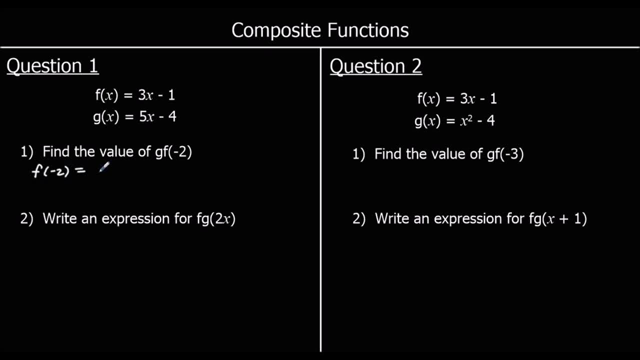 So we've got: g of x is 5x minus 4.. We want the value of g, f of negative 2. So f of negative 2 is 3, lots of negative 2 minus 1.. Negative 6 minus 1 is negative 7.. 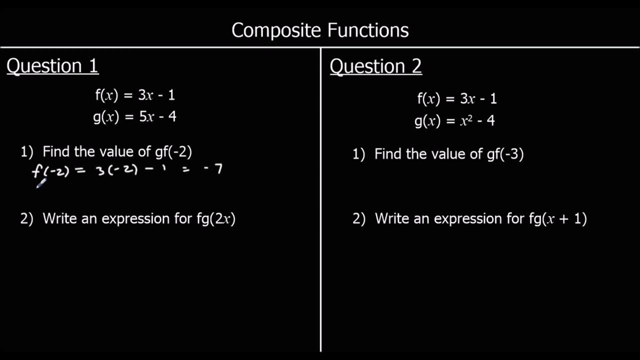 So we're putting negative 7 into g, So g of negative 7 is 5 negative 7s, Which is negative 35 minus 4 negative 39.. And question 2.. Write an expression For f, g of 2x. 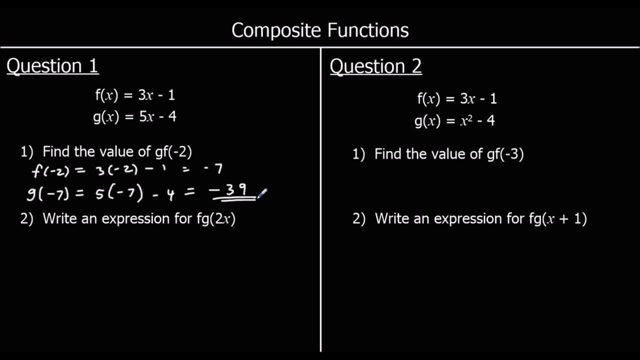 So we're putting 2x into g And then that answering to f. So g of 2x Is 5 times 2x minus 4. Which is 10x minus 4.. Now we're going to put that into f. 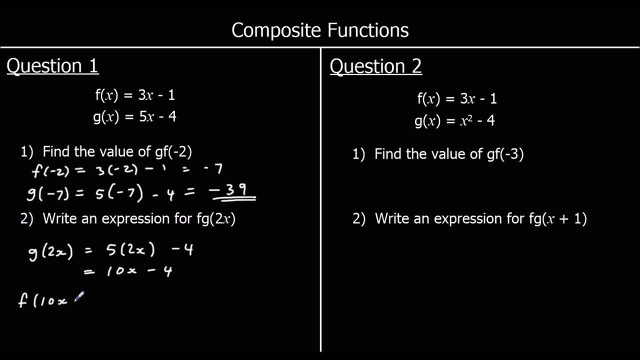 So we're doing f of 10x, Which is 10x minus 4. Which is 3, lots of 10x minus 4. Minus 1.. So 30x minus 12 minus 1., Which is 30x minus 13.. 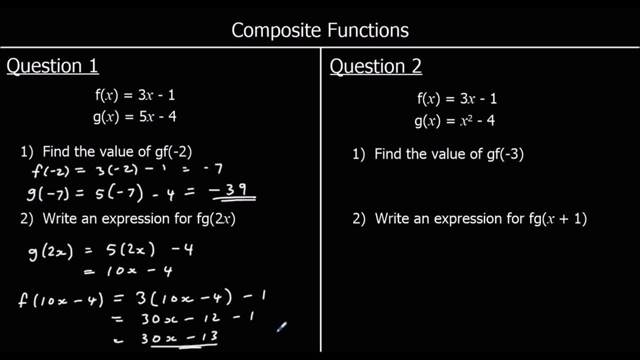 Question 2.. First question: Find the value of gf of negative 3.. So negative 3 into f. f of negative 3 is 3. lots of negative 3 minus 1.. Negative 9 minus 1 is negative 10.. 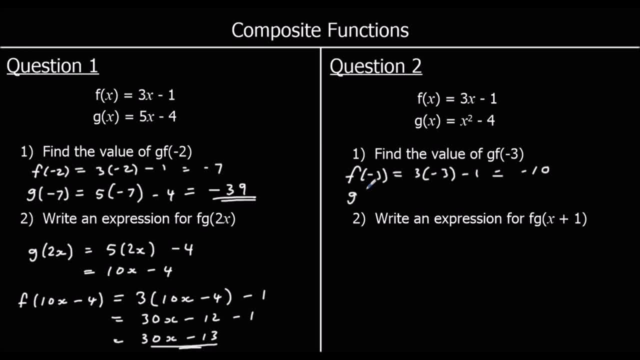 And then we're putting that into g, So g of negative 10. Which is going to be negative 10 squared minus 4.. So 100 minus 4. Which is 96.. And the second question: We're putting x plus 1.. 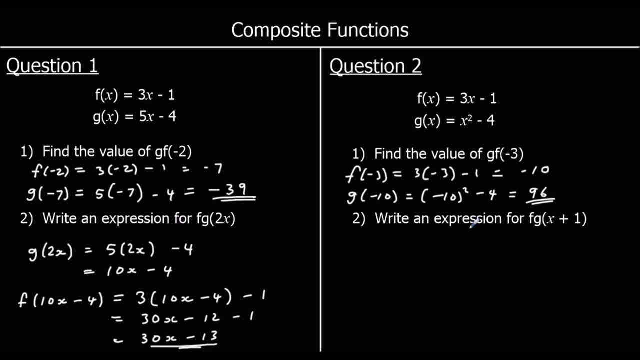 Into g And then that answering to f. So we're putting x plus 1 into g. So g of x plus 1. Is going to be x plus 1 squared minus 4.. So that's x plus 1 times x plus 1.. 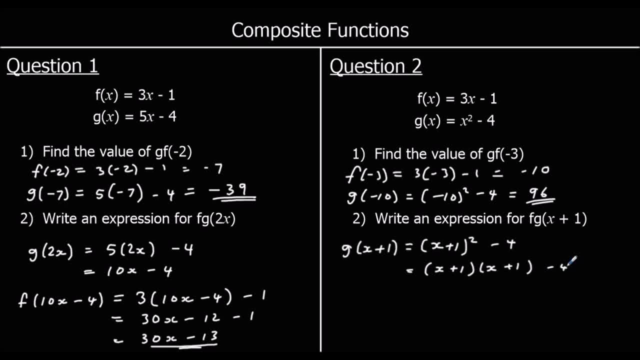 Minus 4.. So we're expanding the double brackets. So x times x is x, squared x times 1 is x, 1 times x is x And 1 times 1 is 1.. So collecting the like terms: 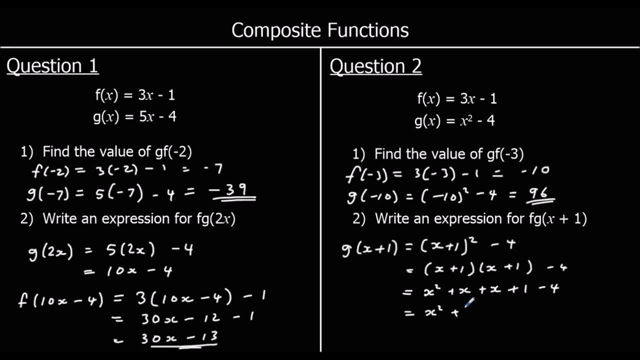 We've got x squared Plus 2x Minus 3.. So that's g of x plus 1. We're going to put that into f, So f of x squared plus 2x minus 3. Is going to be 3, lots of x squared. 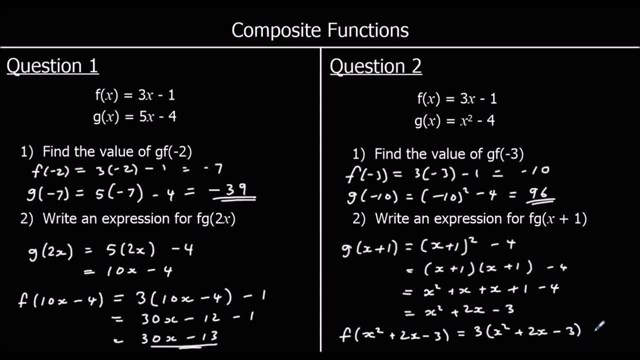 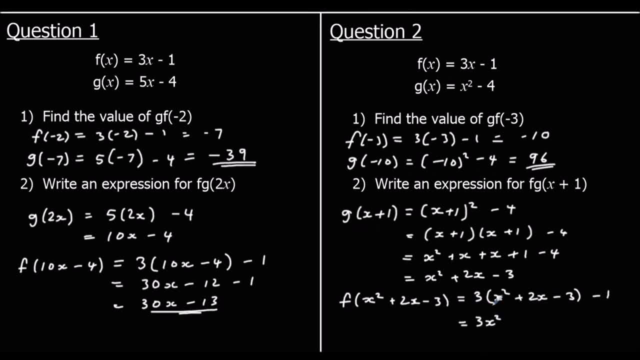 Plus 2x, minus 3. Minus 1.. So that is 3x squared. We're expanding this bracket, So multiplying all of the terms by 3.. Plus 6x, Minus 9. Minus 1.. 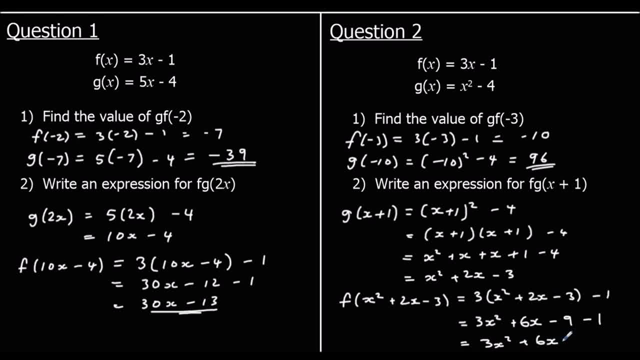 So 3x squared Plus 6x Minus 10. And that is our answer, Thank you. 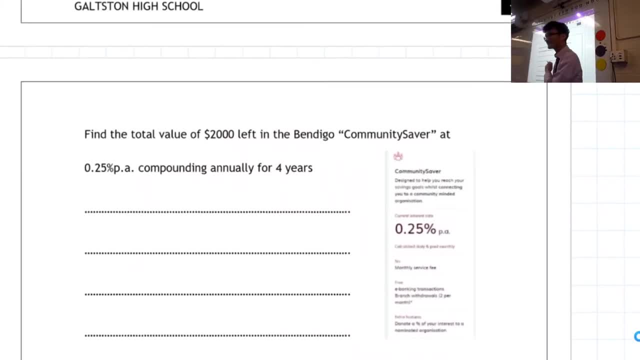 Let's have a look at this one right here. Saxon, can you read it out for me? What have we got? Yep, okay, so often what they do is they give you these problems and they just pluck them out of thin air. 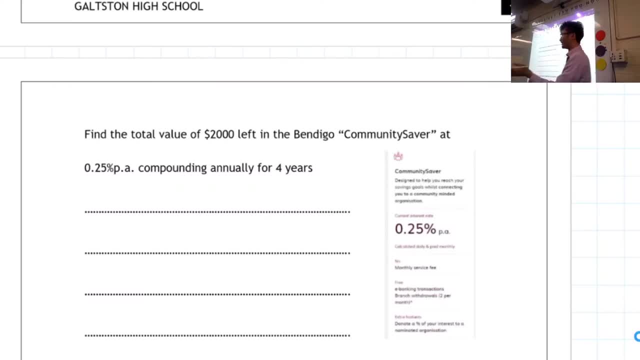 they pluck them out of a textbook or something like that and they say: here's the money you've got, here's the interest you have, and calculate it for me. I always think that's a bit disingenuous, not really real, right. 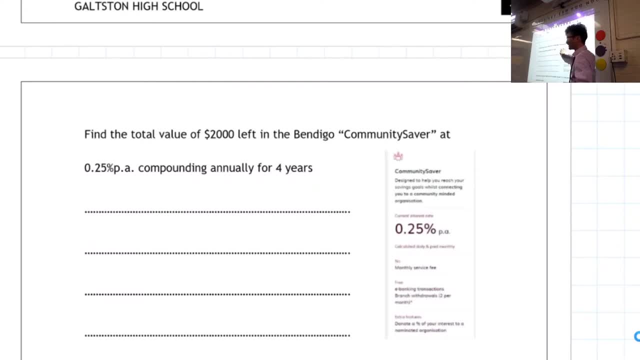 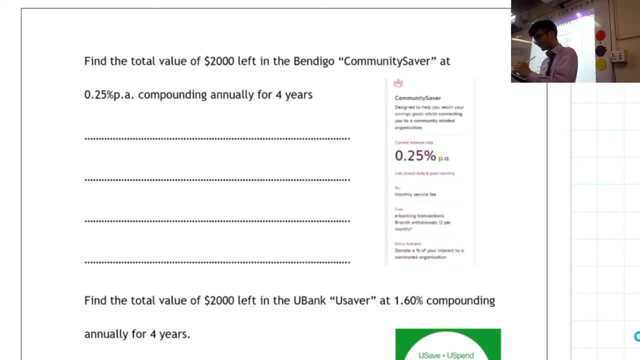 Why would you get these examples from a textbook when you can actually get them from a real place? And here I've picked up the Bendigo Community Saver and this is an actual bank account you can get right Now with the Community Saver. Bendigo Bank is really well known for their accounts that give back to the community. 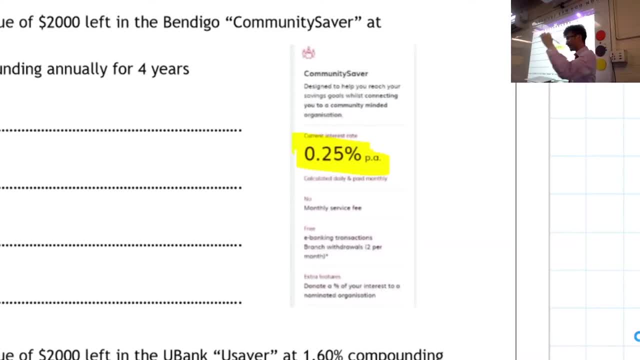 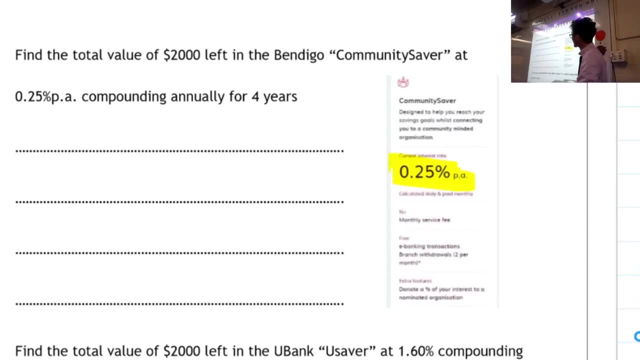 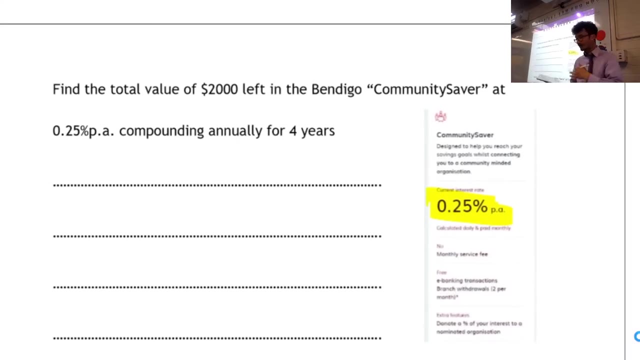 like us. we're like recipients of that right. A lot of the stuff that we have is from the Bendigo Bank. So what I want to do is: how do we approach these kind of problems? Well, we want to Luke, identify all the information. 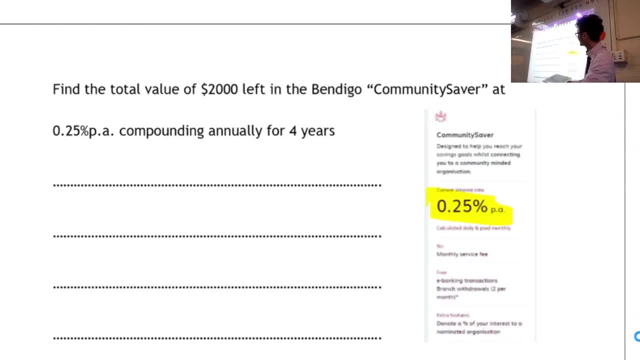 So what information do they tell us here, Luke? The years, Sorry, The years, yeah, good, The value of the 2000.. Yep, that's yep, And 0.25 per annum. 0.25 per annum.